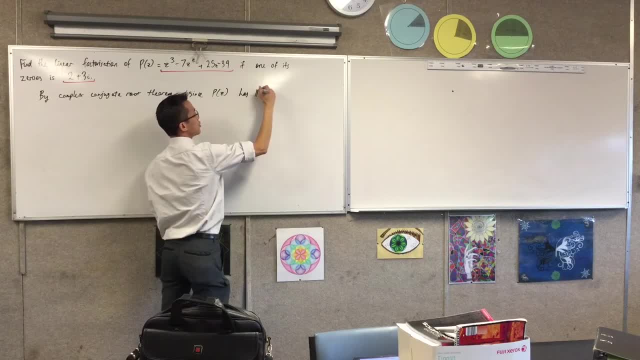 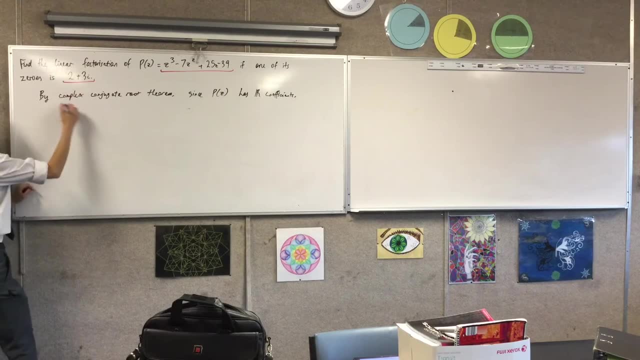 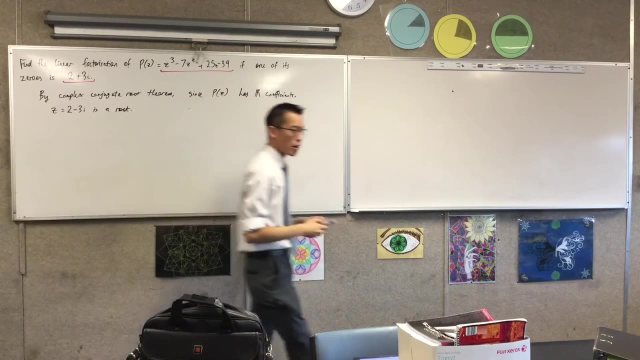 Since P of Z has real coefficients. That means, if I just take the conjugate of this, I've got another root. Okay, now this is great for two reasons. Number one, thinking back to not the free trade agreement, but the fundamental theorem of algebra. this is a polynomial of degree three, which means it has how many complex roots. 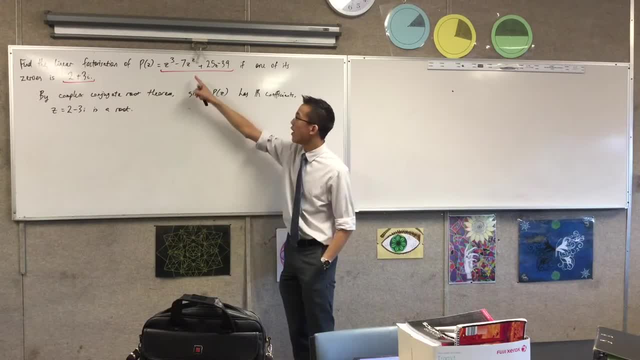 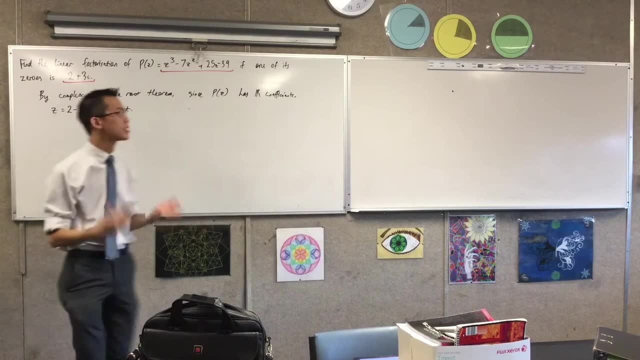 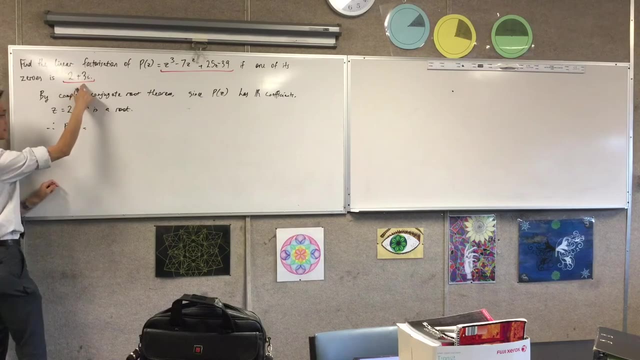 Three, Exactly three, right? No fewer, no more. So I've already got two of them. I only need to find the last one That'll be useful to me in this class. Okay, so now that I know these two, that tells me something about the factorization, right. So I can say, therefore, P of Z is equal to: I've got Z minus this, Z minus that, and then I'm going to have some quotient along the end, okay. 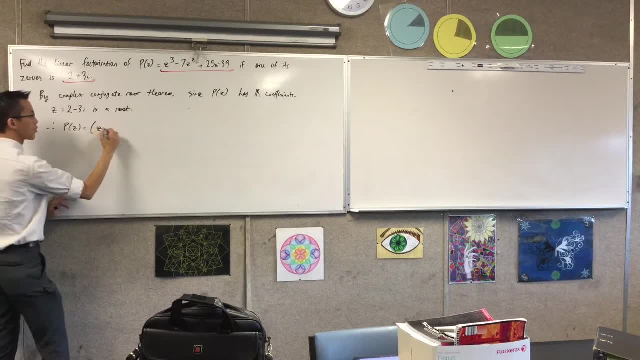 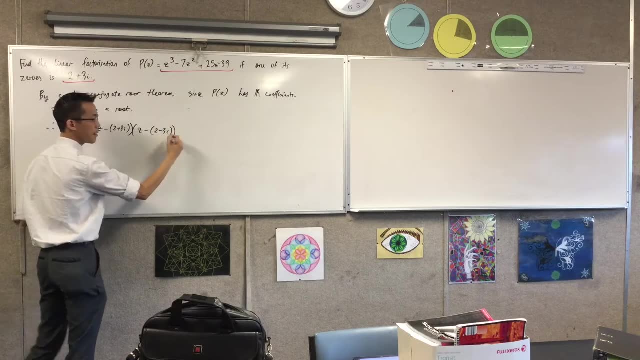 So I'm going to have just watch out your brackets and signs here. I'm going to write it as Z minus this, Z minus this, So you can't actually just solve two plus three. I into the equation? Oh, because it's a linear equation. 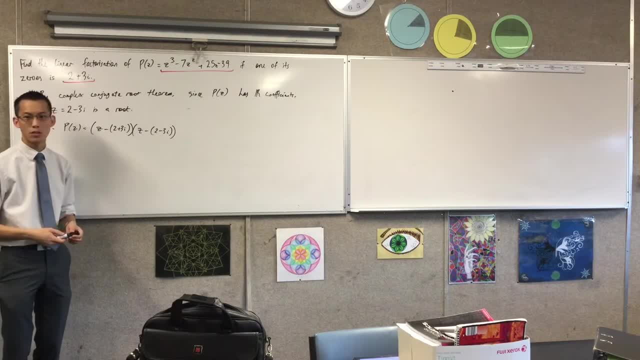 It would be just a linear equation. I can, I can, but it won't give me anything useful. All it will tell me is zero according to the factor theorem. right, Like it will just pop in and say, yep, it's right. That's all it will tell me, okay. 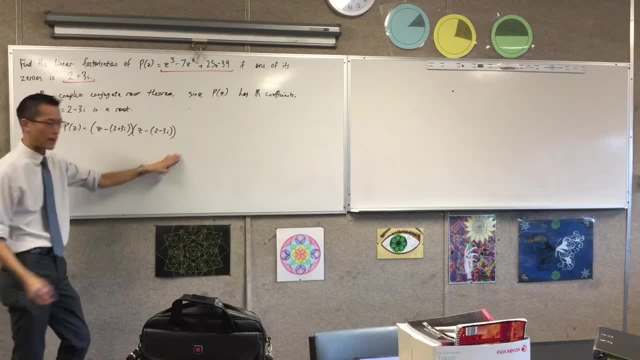 So there's the first two factors that I already know. Now I don't know what the other factor is. I'm just going to call it Q, partly because I already have P and Q for quotient. okay, because having divided, divided is fair. 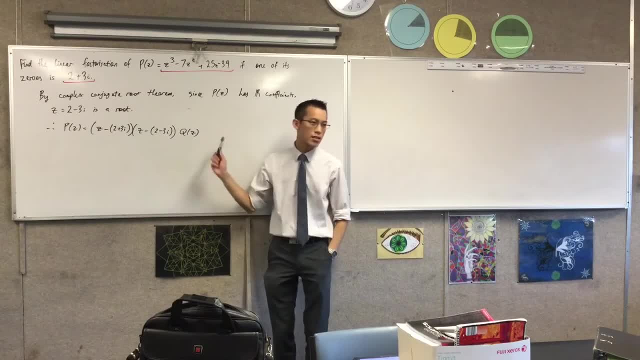 Now have a look at this. What I want to try and get to is: well, what's the final factor? Because I want a linear factorization, like we said. So, degree three: I've got one. two, that's the third one, okay. 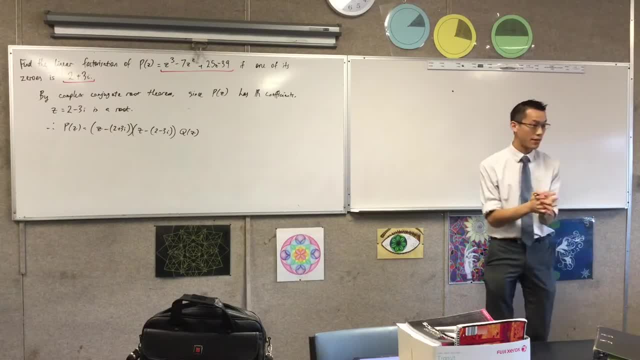 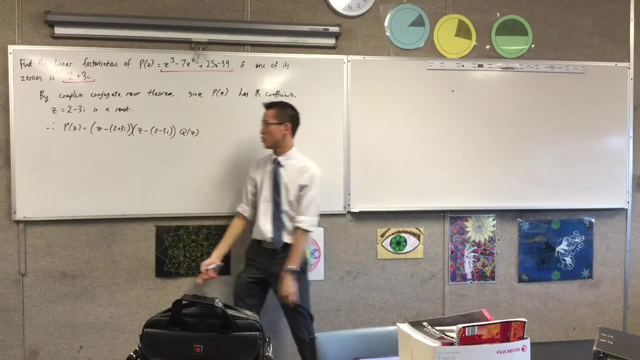 Before I get there, you can see, one of the great things about the fact that they're complex conjugates is that these guys are going to simplify out really, really easy. okay Now, before you launch into doing three terms times three terms and end up with nine terms at the end, 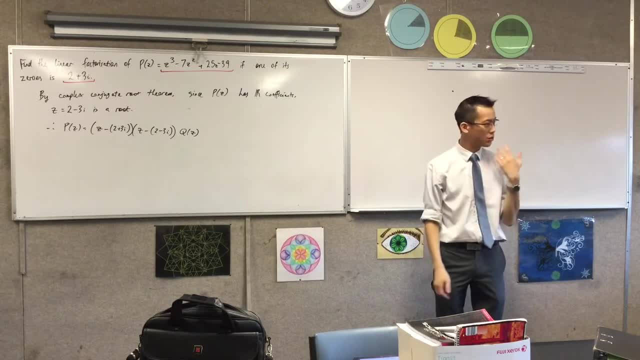 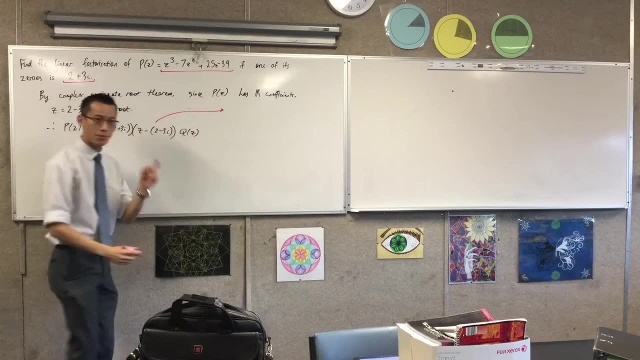 which hopefully will simplify out into your algebra. I want you to remember some of the properties of these complex conjugates, right. So maybe just off on the side here- This is a secondary note- If you have, If you have z minus alpha and z minus alpha bar, okay. 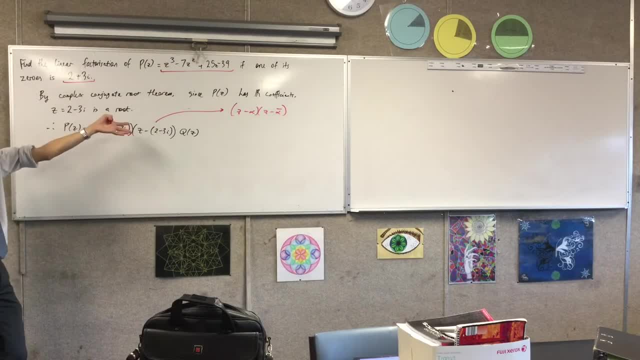 Think about this for a second. Just think about how it's going to expand just as a Come in, Come in, That's right. Just think about how it's going to expand as a binomial. okay, What are we going to get? 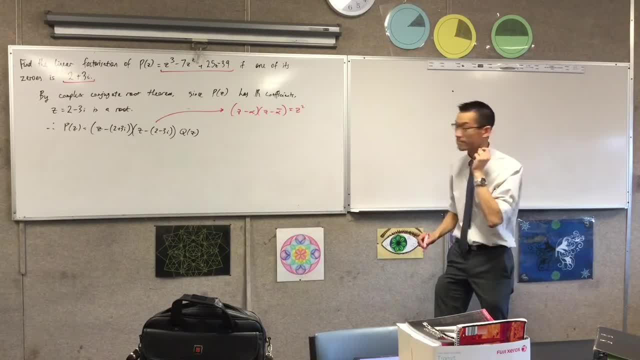 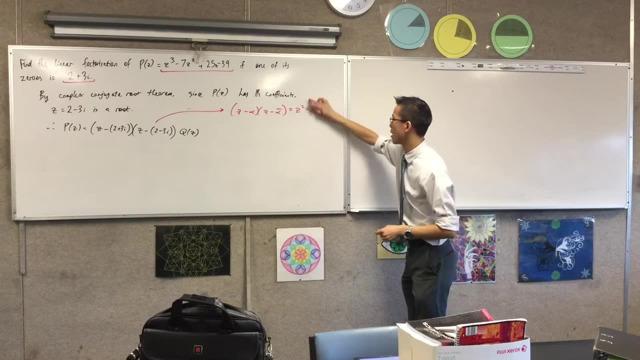 You're going to get z squared out the front, Minus, Minus Alpha z To Oh Sorry, No, I'm sorry, No, I'm thinking of a picture. It's going to be alpha. Just think about how you're going to put them together, right. 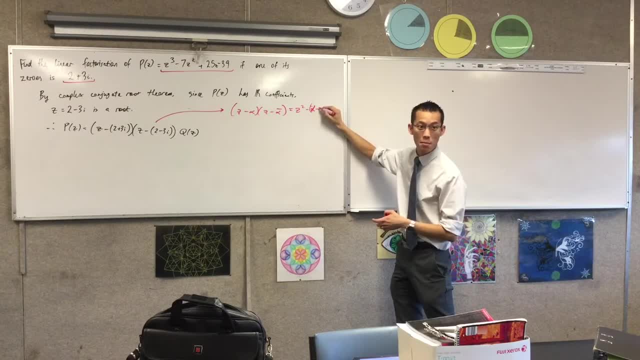 So if I say alpha z, it's going to be also an alpha bar z right. And then what's trailing along on the end? It just comes from the constant term right, Which is plus alpha, alpha bar, Is that okay? 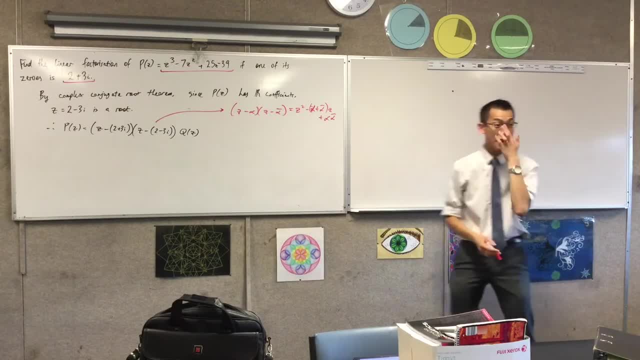 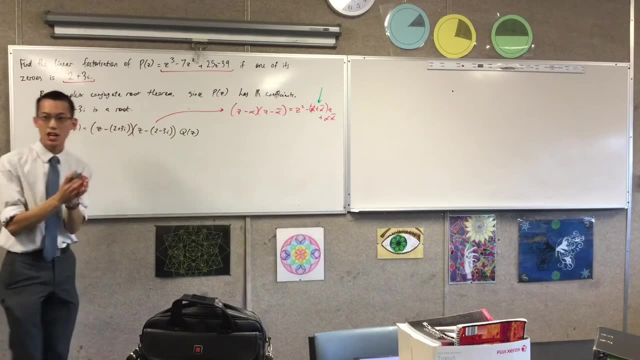 But remember what alpha and alpha bar are and how they relate to each other, right? They are complex conjugates. So therefore, Another color. When you add them together, When you add them together, The imaginary parts are going to disappear or they're going to cancel out, right? 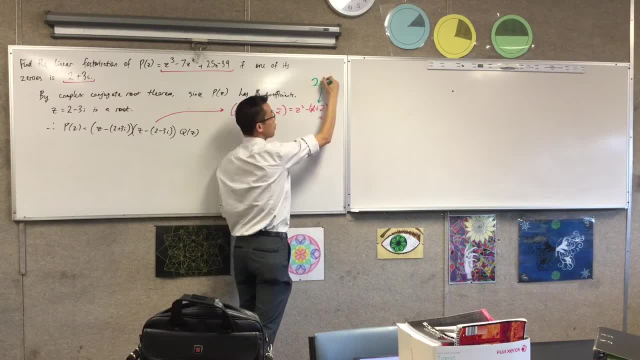 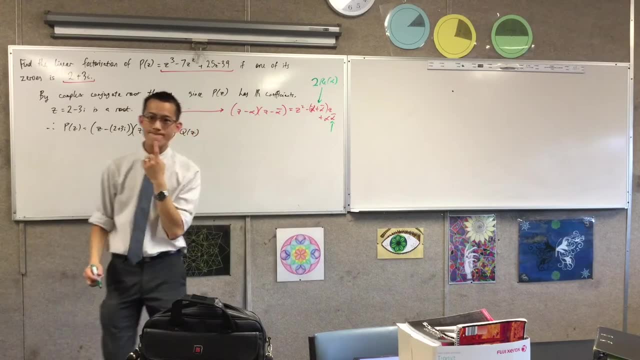 So, in fact, all you're going to get is two lots of the real part of alpha. Do you agree with that? Right, The imaginary part will disappear. Okay, what happens when we multiply them? Hmm, What happens when you multiply them? 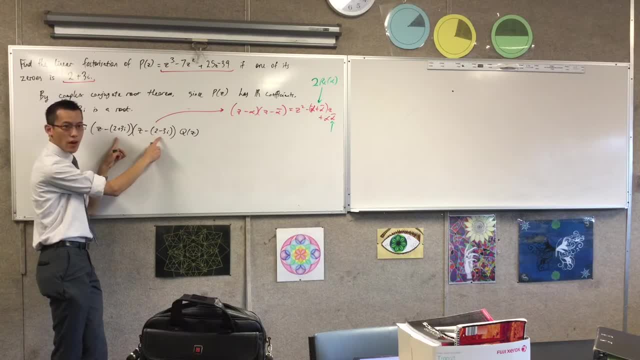 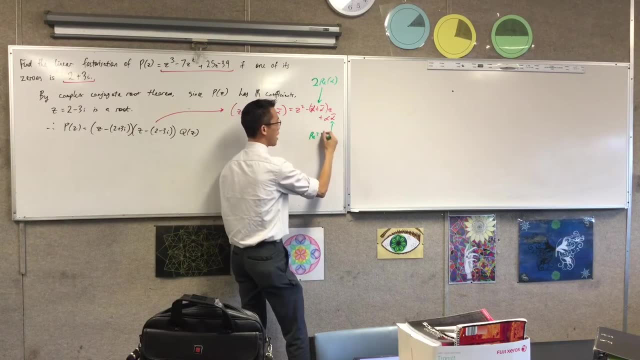 Look at them. Look at what's going to happen. It's difference of squares, but because of the i's that come in, it ends up being the sum of squares, right? So in fact, this part is going to become the real part of alpha squared. 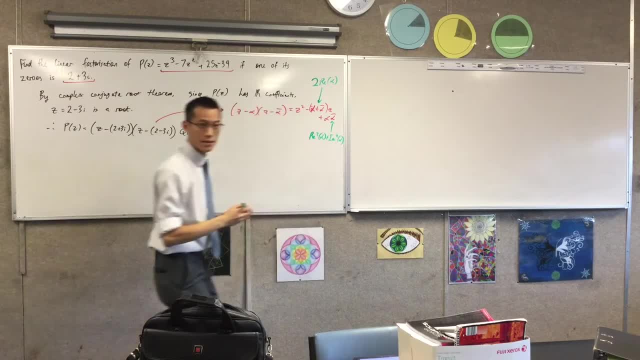 And the imaginary. It's going to become the imaginary part of alpha squared. Okay, Does that make sense? And that's going to dramatically make this simpler. Like every time we use the complex conjugate root theorem, we're going to get complex conjugates. 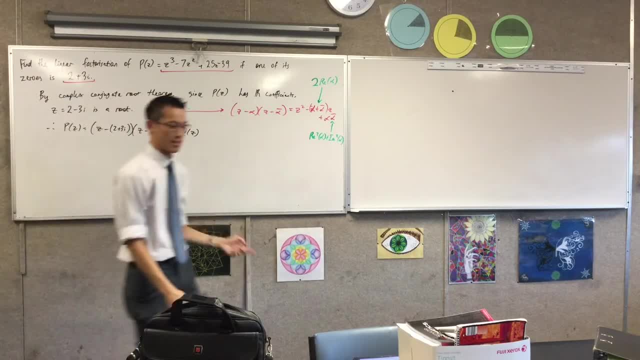 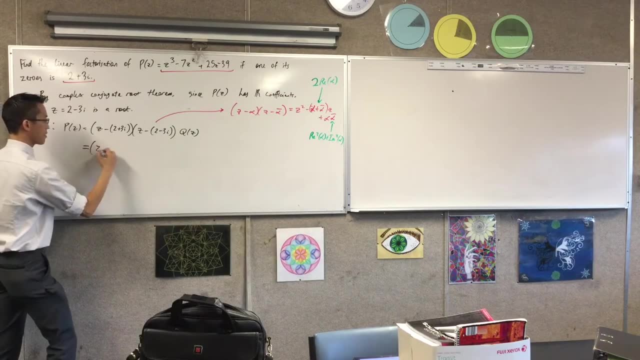 So, rather than multiply this whole thing out- it's a disaster and you're asking for silly errors to creep in- I'm just going to take advantage of these results. So, for instance, I'm going to get it quadratic, as I know, right. 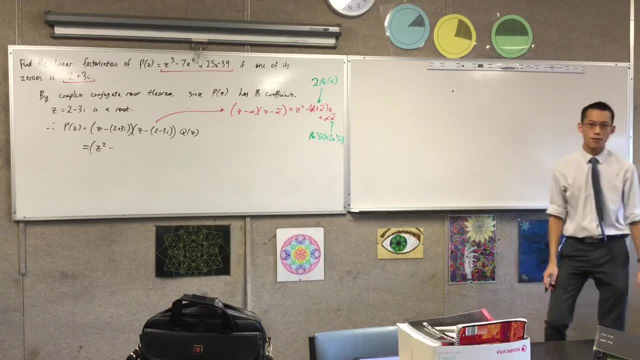 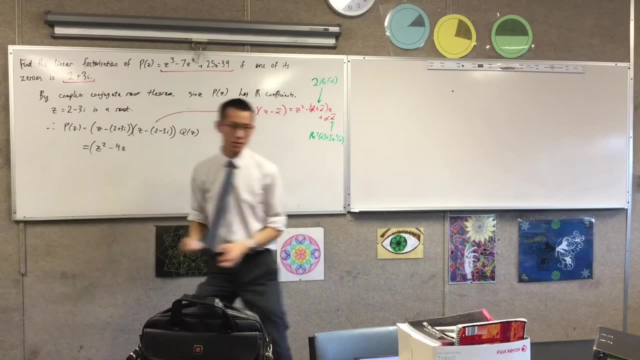 And then I'm going to take away. Now, what's double the real part of my chosen alpha? Yeah Well, the real part is just 4.. Gee, that was a lot simpler than trying to deal with the three terms that are going to be the zip term, which would be a mess. 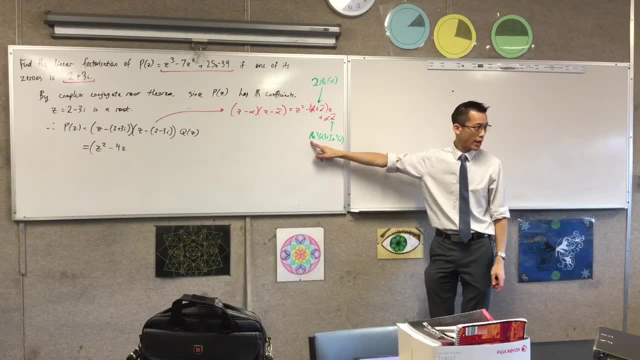 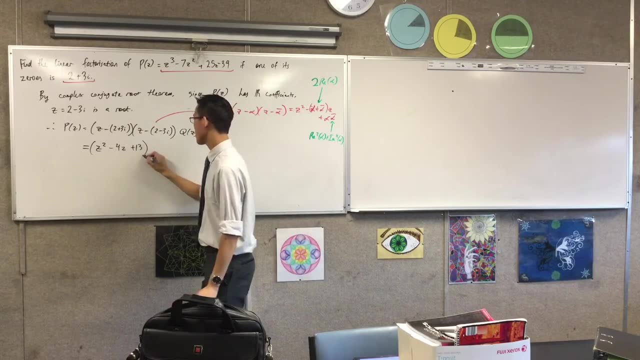 And then I'm going to add on the real squared and the imaginary squared. That looks like 4 and 9 to me. Yep, So that's 13.. Whoa, Just like that, Right? This is why complex conjugates are so easy to work with. 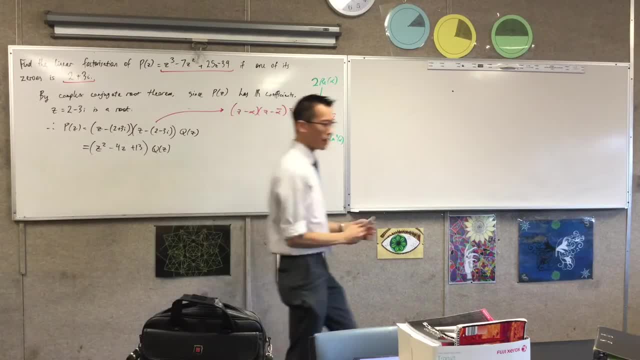 Okay, Does that look right? Yeah, Looks good to me. Okay, So at this point, there are one of two things that we can do. There are two paths to finish out the question and find out what this Q of Z is. 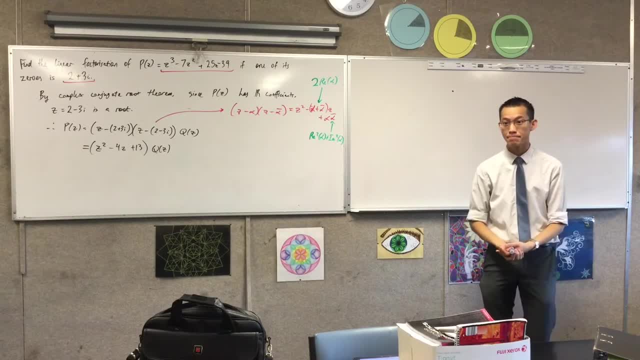 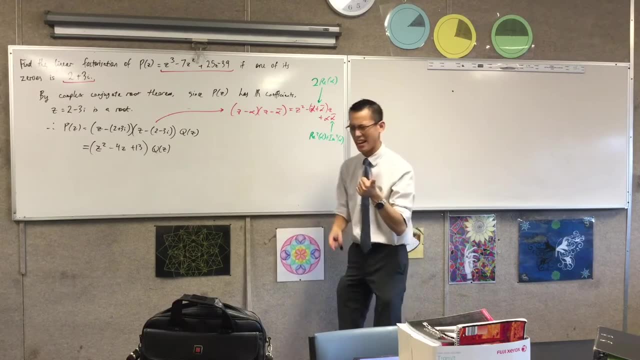 Anyone want to suggest to me what one of the paths might be? Look at the constant term and say you need 3, get 39. Okay, So the first method is. The first method is- And I need to actually rewind a little bit- right. 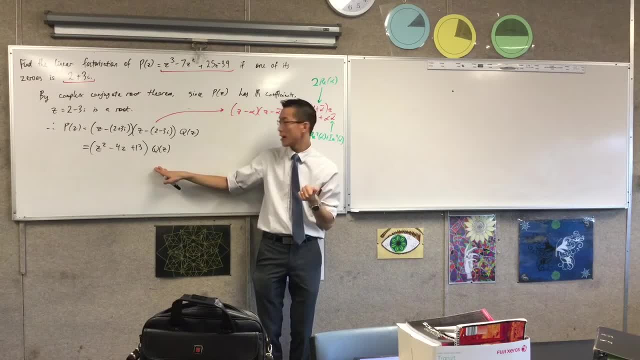 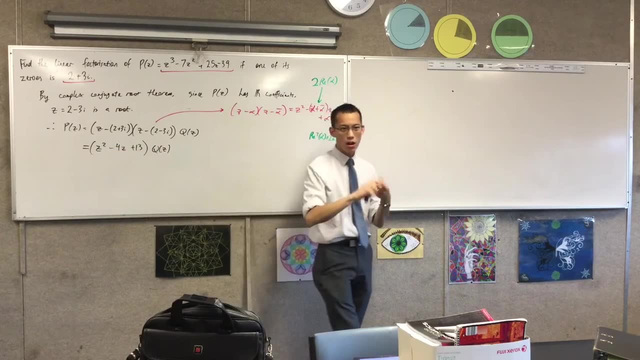 The first method is to recognize: okay, this must be a linear factor. right, It must be linear, because I've already got degree 2 here. This has to multiply to degree 3. So this must be degree 1. It's not only linear. 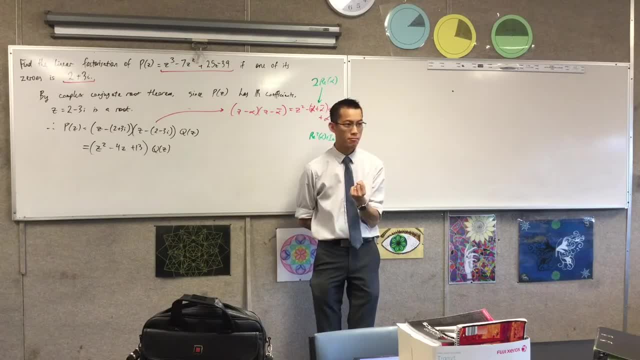 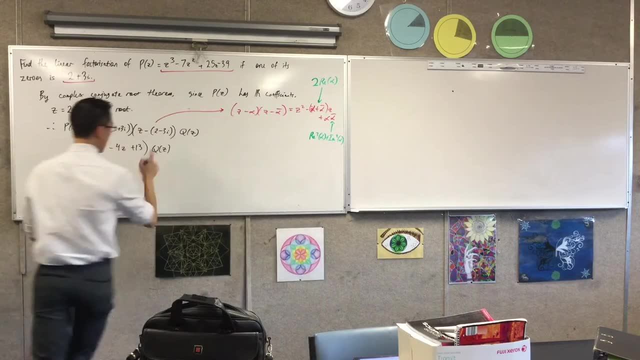 I also know it's monic. How do I know it's monic? This is monic, This is monic. That must be monic. Okay, So it's got to be monic and linear, which means that I can write this in this form: 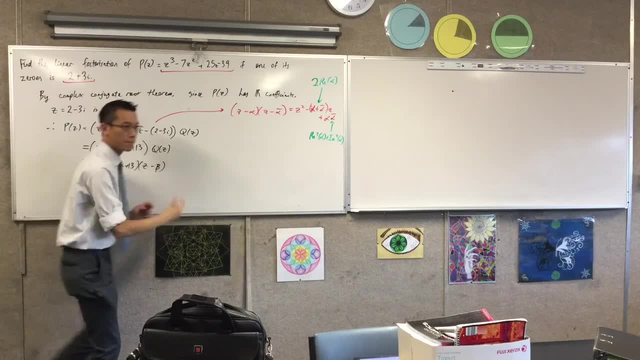 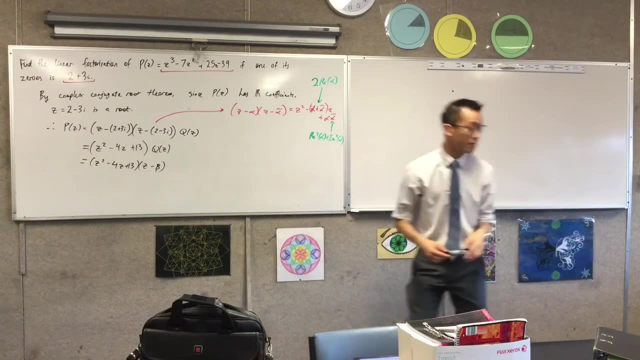 Z minus. I already talked about alpha, so I'm just going to call that here. Okay, Yes, It has to be real as well, because if it was a complex number, it would make a number like this: Yes, Very good. 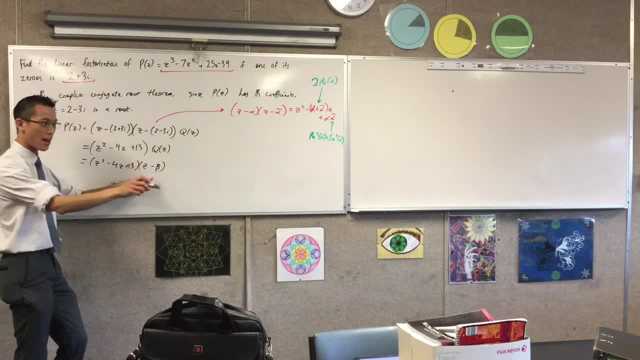 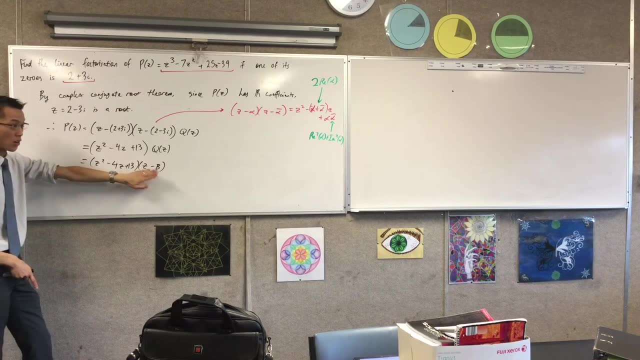 It would have. Yes, that's right. So, in order to have like the issue you're talking up against, is the complex conjugate root theorem right? I know that either you're going to have conjugate or you're going to have complex coefficients up here. 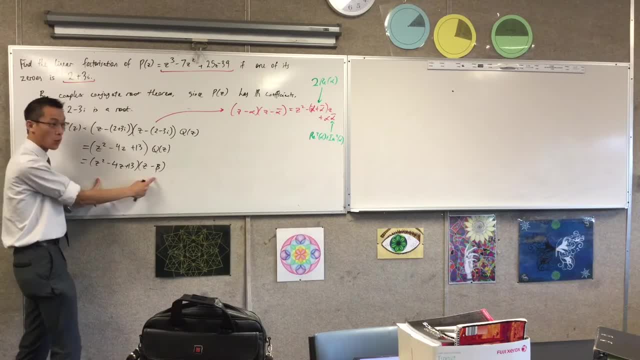 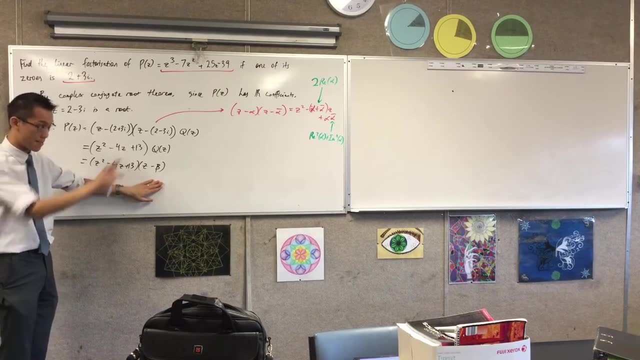 And I can't have either of those right Because I've already used two of my roots. I've only got one left And I don't have any complex coefficients to get an extra thing out of. So that's nice. I don't necessarily need to state that, but it's helpful to know, okay.